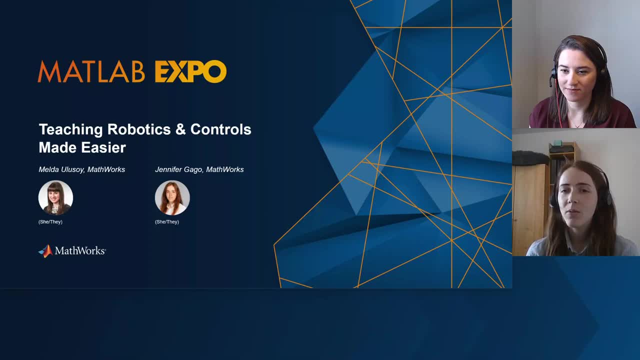 who works in the Matworks Academy group. In this session we are going to highlight various tools and resources for educators teaching robotics and controls, including downloadable coursework materials, interactive examples, virtual labs and much more. First, Milda will focus on the theoretical part of teaching robotics and controls. Later I will talk. 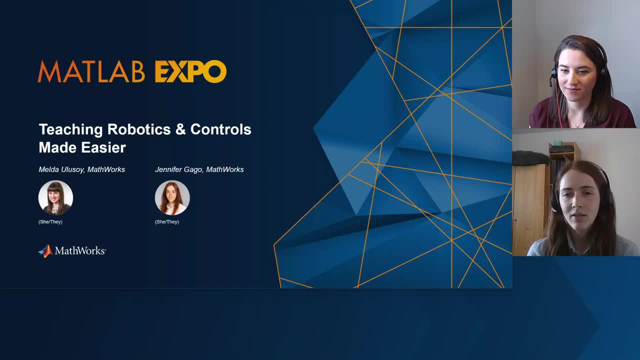 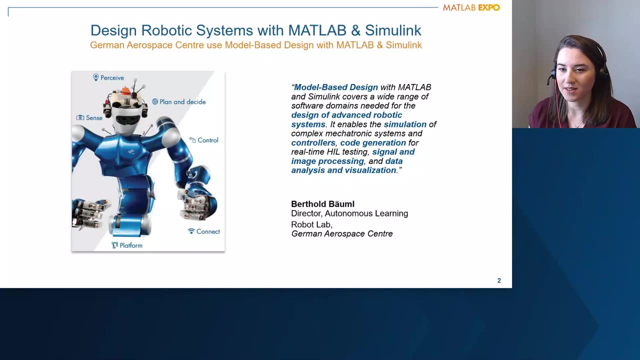 about the practical aspects of it. You can download the presentation slides from the hands-out section and, alternatively, you can access them on the Expo website. Designing robotic systems is a multidisciplinary task that involves perception, sensing, planning and decision, platform use, connectivity and control. 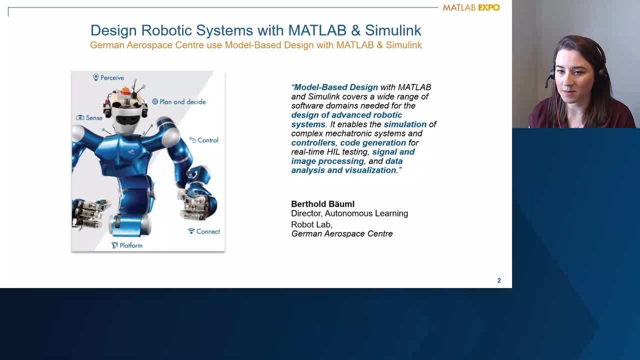 To successfully design and develop robotic systems, we need tools that allow us to effectively cover all these areas. The director of the Autonomous Learning Robot Lab highlights MATLAB and Simulink to design advanced robotic systems, which includes design and simulation of controllers, automatic code generation and data analysis and visualization, among others. 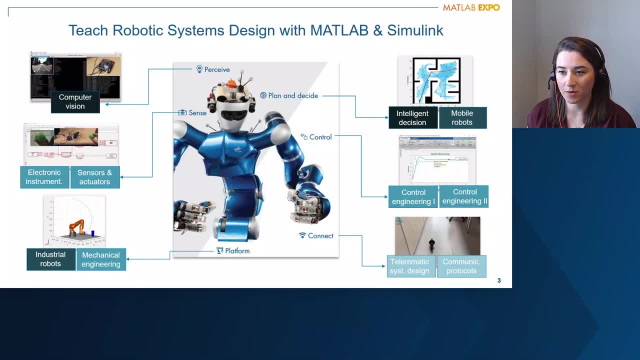 Teaching robotics engineering requires a multidisciplinary approach reflecting the needs of the students so that they can easily develop robotic systems. The courses offered in the course are more complex and more flexible than the wide range of courses offered in a typical program. However, this can pose a challenge for instructors when 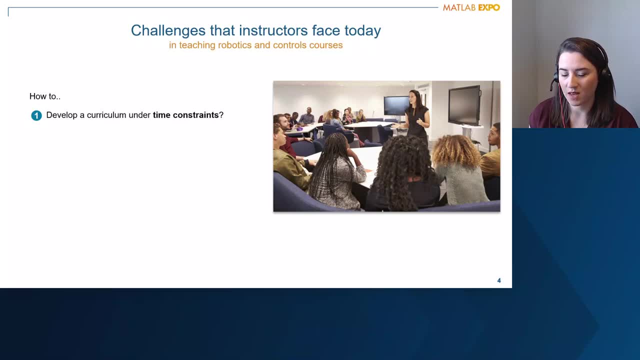 designing content and activities for students. Therefore, this presentation will explore various tools and resources that can assist instructors in delivering a comprehensive robotics degree with an emphasis on controls. One major challenge is time constraints, that many of you might have experienced when developing a curriculum. 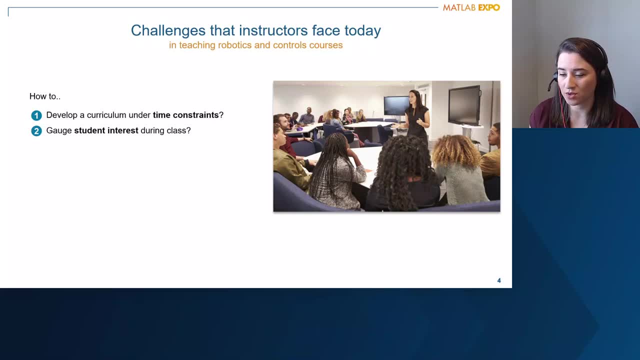 Other challenges include to keep students engaged during class and find ways to facilitate independent learning. Hands-on learning is crucial for students as it lets them to apply their learnings from class to real-world applications. However, it can be challenging to scale access to resources for hands-on learning. 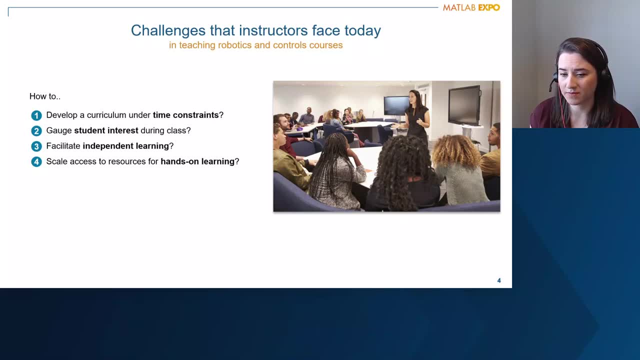 Especially when it comes to hardware resources. Grading student assignments and providing constructive feedback can also be difficult, particularly with a large number of students. Finally, it is important for instructors to provide opportunities for students to work on projects that push the boundaries of their understanding. 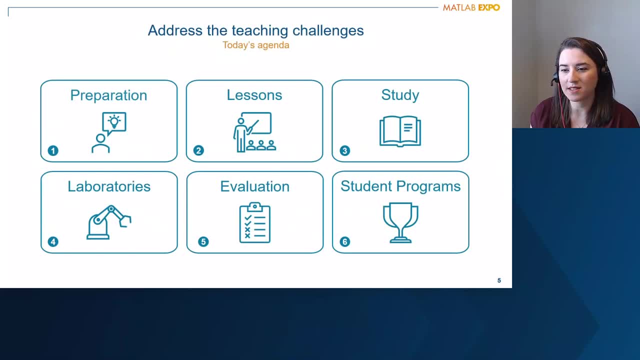 To address all these challenges, we designed an agenda that incorporates different teaching activities, with each activity focusing on a specific challenge and proposing a corresponding solution. We will first start with preparation of the classes, where main challenge is developing curriculum under time constraints. In this section, we will discuss how you can use ready-to-use courseware to save time during course preparation. 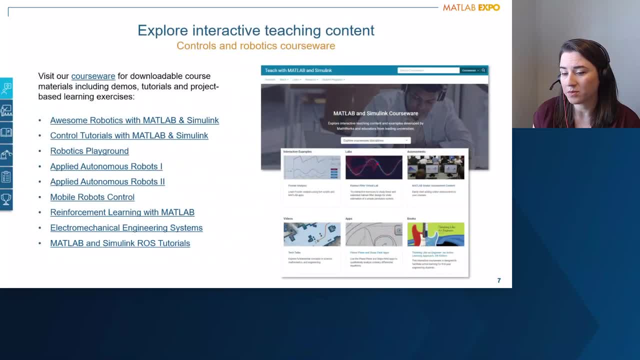 Whether you are putting together a new curriculum or want to enhance your existing one. we will also discuss the different teaching content that we have available on the MATLAB and Simulink courseware site. Resources you will find here are tailored to multiple disciplines, including robotics and controls. 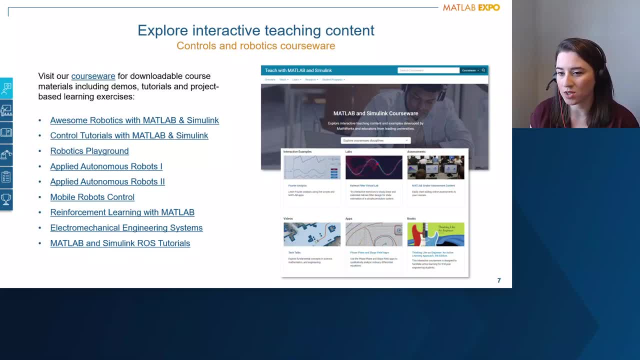 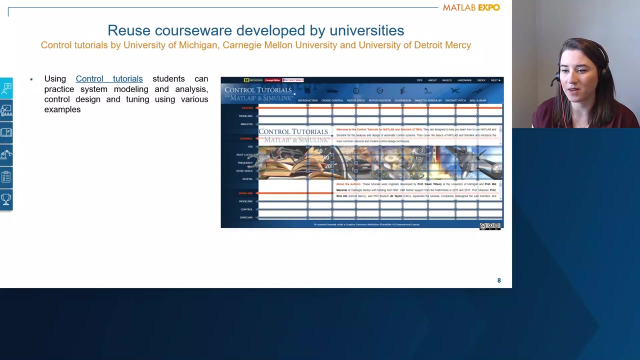 and include downloadable course materials, virtual labs, educational videos, apps and project-based learning exercises developed by both MathWorks and faculty from leading universities around the world. Next, we'll take a look at one of these teaching materials. There are many great curriculum materials developed by universities. 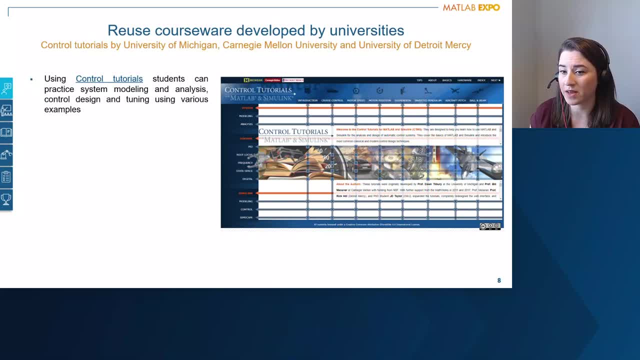 and shared broadly with the community to be used by instructors as well as students. Such an example is the Control Tutorials with MATLAB and Simulink developed by University of Michigan, Carnegie Mellon University and University of Detroit, Mercy, in collaboration with MathWorks. 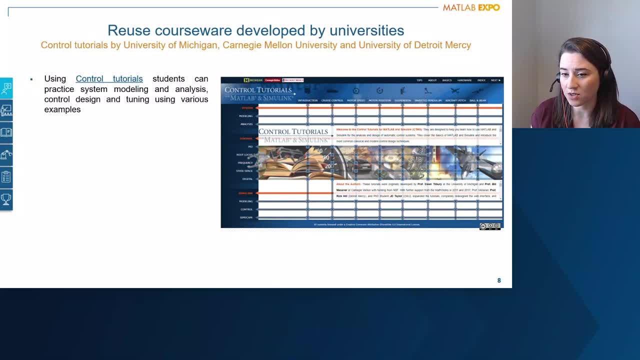 These tutorials facilitate self-study, self-instruction on various controls topics, as well as the use of MATLAB and Simulink. You'll find a range of Common Control System related examples, and for each of the examples you'll find tutorials on system modeling and analysis. 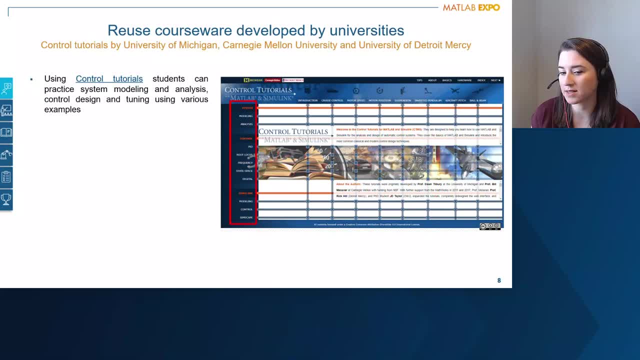 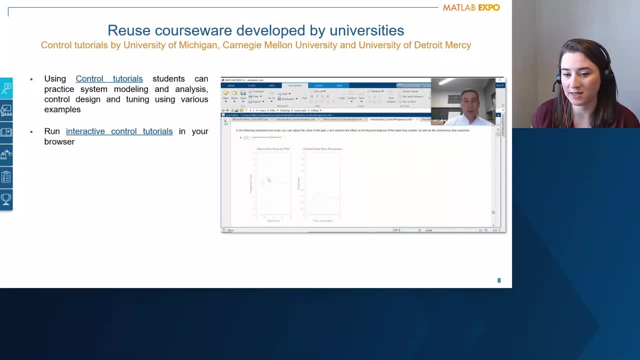 control design using PID, root locus, etc. Some of these tutorials are available in MATLAB Live Scripts, which we will discuss later in more detail. The Live Script Control Tutorials lets you interactively update parameters of dynamic systems and immediately see results, as shown in the video clip here. 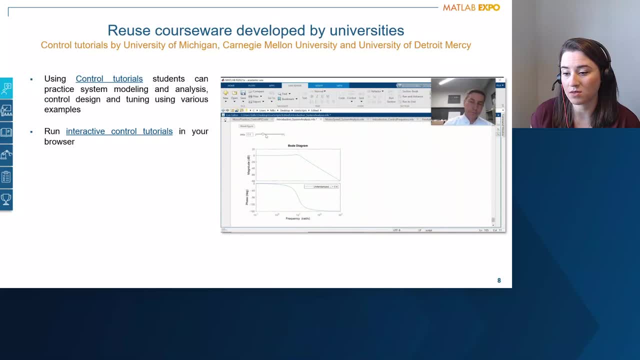 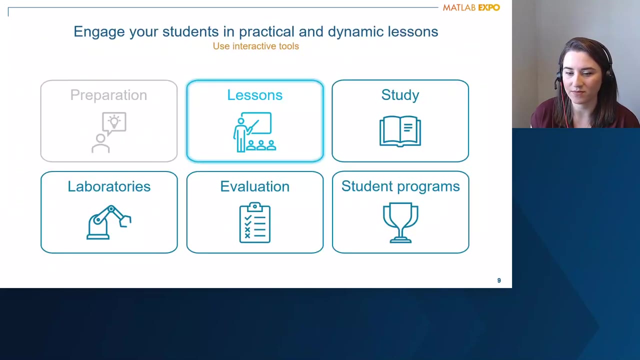 They can also be run in any browser without the need to install MATLAB. To learn more about the Control Tutorials and how to use them for teaching controls, you can check out the webinar by Professor Richard Hill from University of Detroit, Mercy. We will focus on lessons and discuss how to gauge students' interest during class. 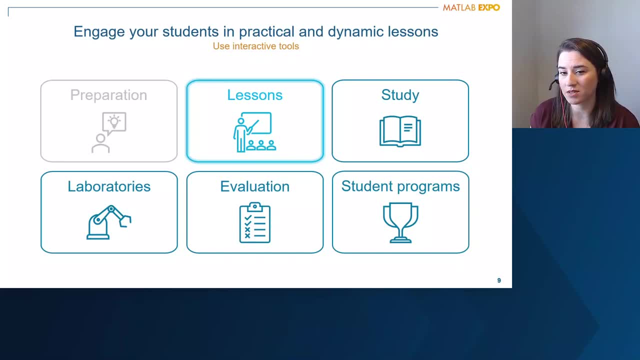 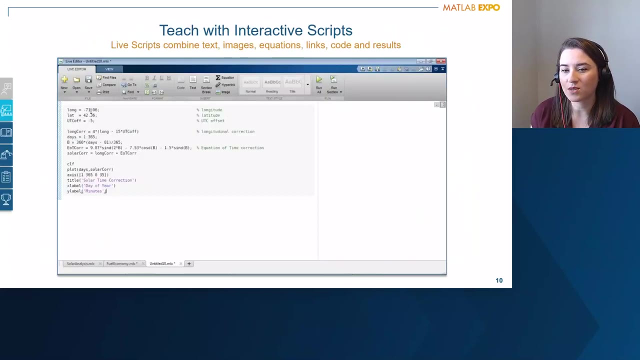 so that they can get the most out of the teaching hours. In this section, we will highlight various tools and resources you can use to make your lessons more engaging and dynamic, encouraging students to actively participate in class. A great way for engaging your students is to use MATLAB Live Scripts. 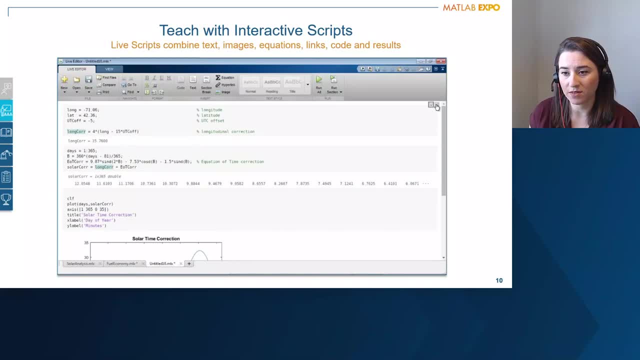 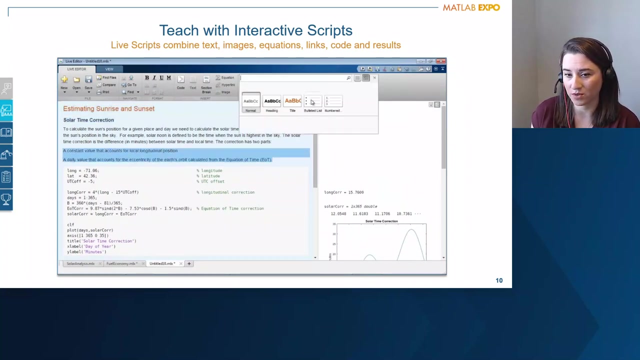 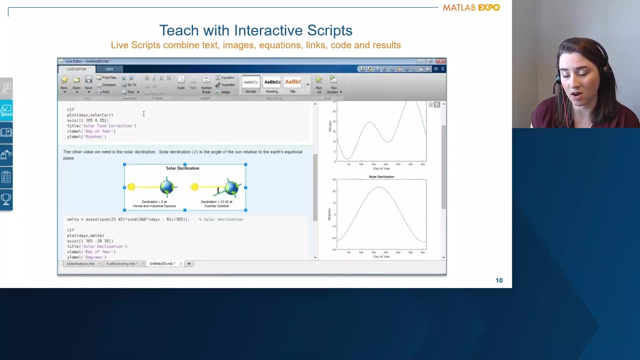 With Live Scripts, you can create interactive lectures by combining code and results with formatted text and mathematical equations. You can also insert images and interactive controls such as sliders, buttons and drop-down menus. You can create step-by-step lectures and evaluate them incrementally. to illustrate a topic: 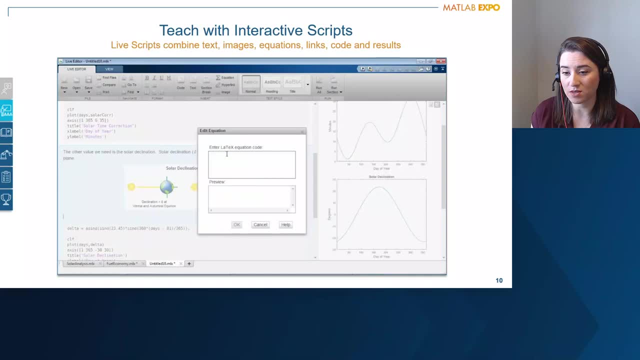 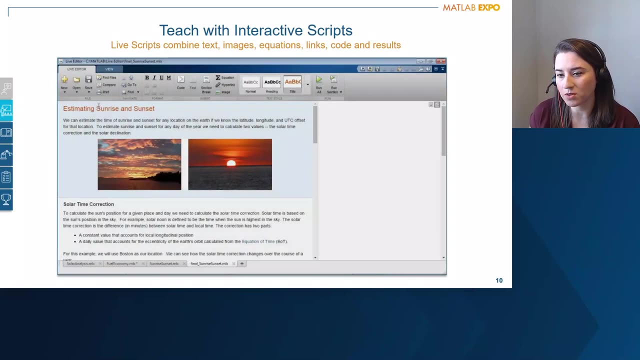 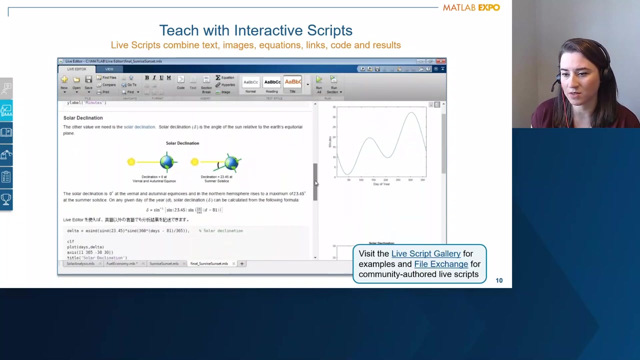 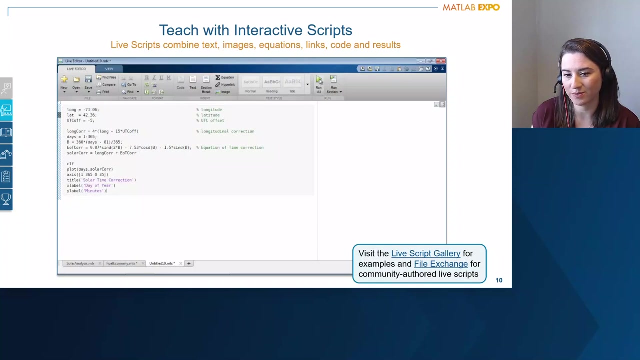 You can modify code on the fly to answer questions or explore related topics, Share lectures with students as interactive documents and distribute partially completed files as assignments. For more examples, you can visit our Live Script Gallery and MATLAB File Exchange for Live Script examples authored by other instructors like you. 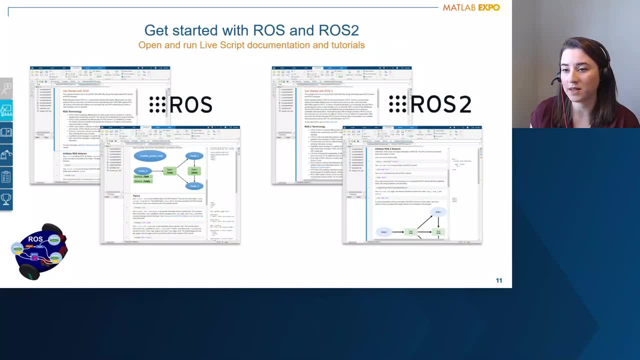 Here we show an example of Live Scripts to explain complex concepts in robotics. The tutorials developed by MathWorks on the use of ROS with MATLAB and Simulink contain Live Scripts that take the form of nine interactive lessons, four hands-on projects and technical documentation. 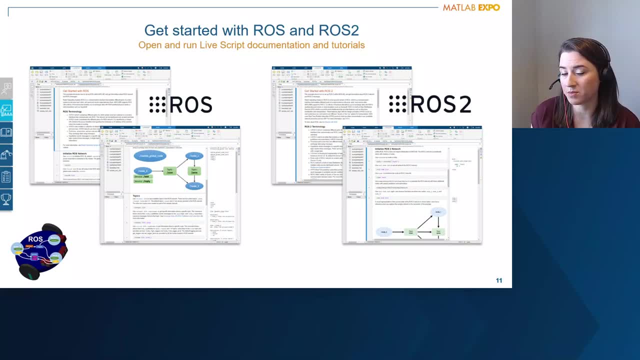 to get you started with ROS and ROS2 in a practical way. The combination of theory with a graphical and interactive component promotes the best assimilation of concepts by the students. We encourage you to try this example, which is available on the MATLAB File Exchange. 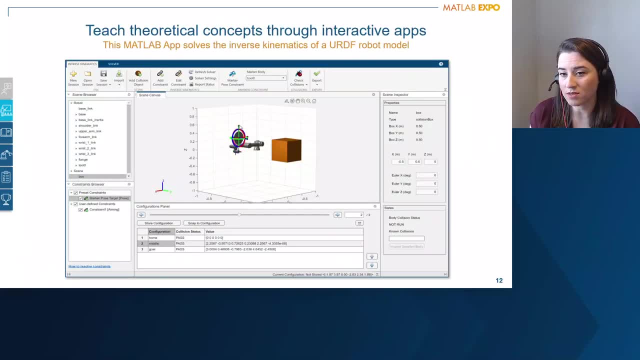 Another tool for engaging students is apps. Teaching with apps allows students to become familiar with new theoretical content in a visual and practical way. With MATLAB App Designer, you can create interactive applications without having to be an expert GUI programmer. Simply drag, drop and resize components and program their functionality. 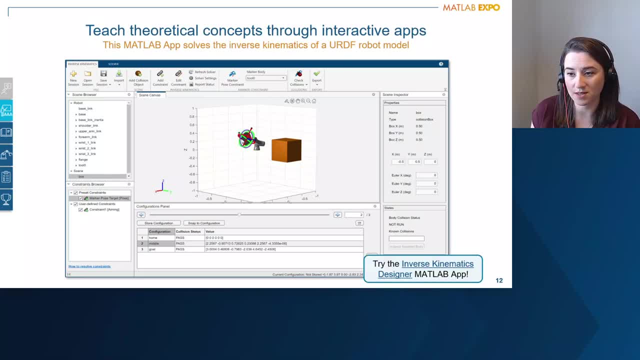 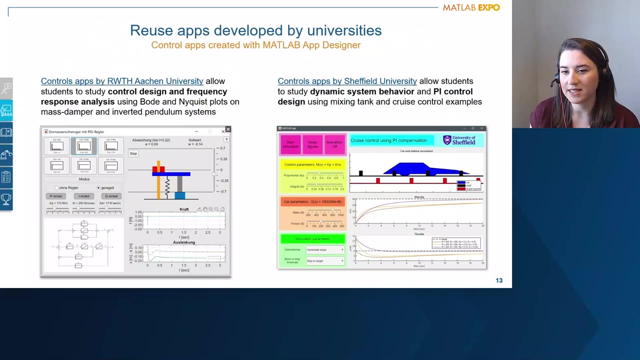 You can find apps designed by MathWorks such as this example included in the Robotics System Toolbox, which shows an application that allows you to calculate the inverse kinematics of a robotic arm by simply modifying its position with the mouse pointer. In addition to apps provided by MathWorks, 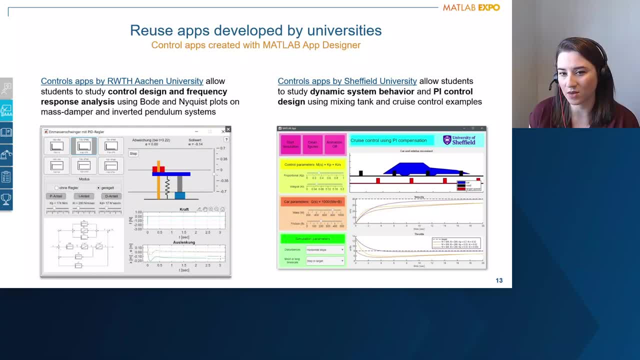 you can also find apps developed by instructors like you. On the left you see an app developed by RWTH Aachen University to visually teach control design and frequency response analysis of systems such as mass tamper and inverted pendulum, And the picture on the right highlights apps developed by University of Sheffield. 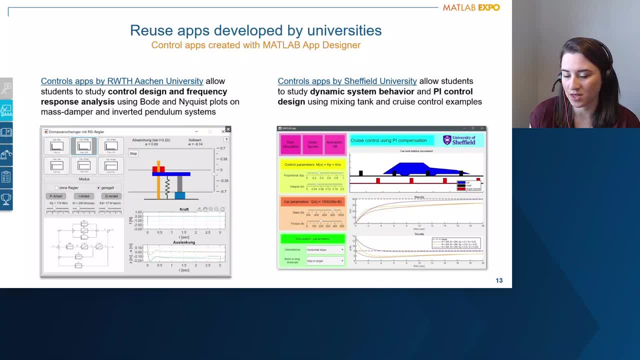 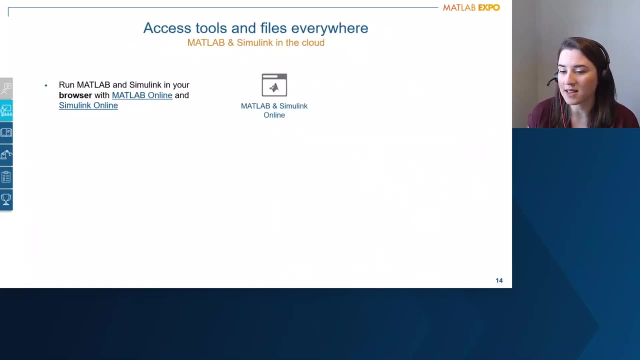 to teach fundamental topics in controls such as dynamic system behavior and PI control design. You can find and download these apps using the provided links on the slide. Once you have interesting examples to show in class, you can facilitate their use by students by leveraging MathWorks' cloud-based tools. 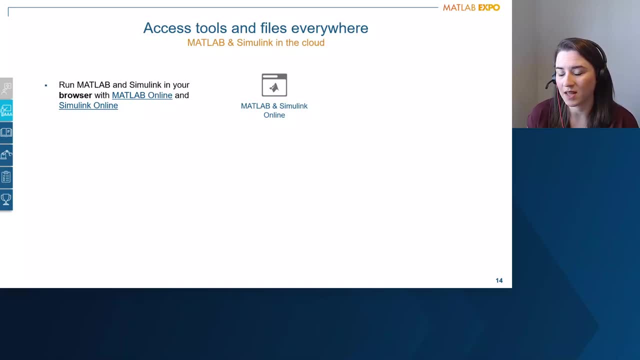 such as MATLAB and Simulink Online. With the online tools, you can run the latest version of MATLAB and Simulink in your browser without the need for downloads and installations. With MATLAB Mobile, students can follow along instruction on their mobile devices. 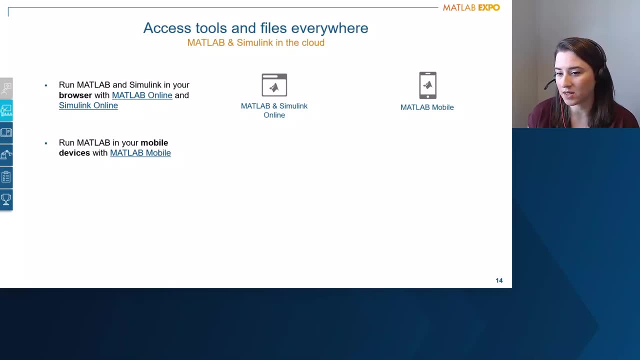 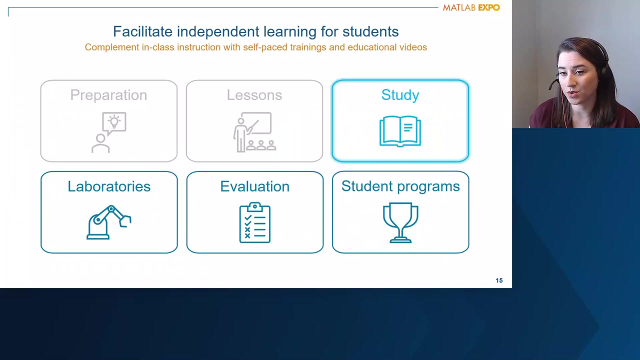 They can create, edit and run scripts and instantly connect results to concepts they're learning. You can collaborate and share files with students thanks to the 20 GB of cloud storage provided by MATLAB Drive. Now that we've seen various tools and resources to prepare and conduct our theoretical lessons, 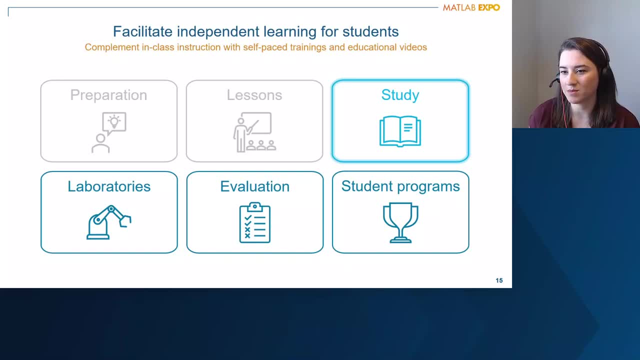 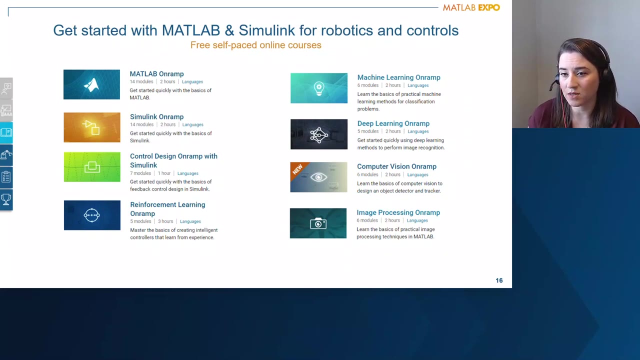 let's see how we can facilitate the study of these subjects for our students. In this section, we will highlight online courses and educational videos for self-learning of robotics and controls concepts. OnRamps are free self-paced online courses that students can take to get started. 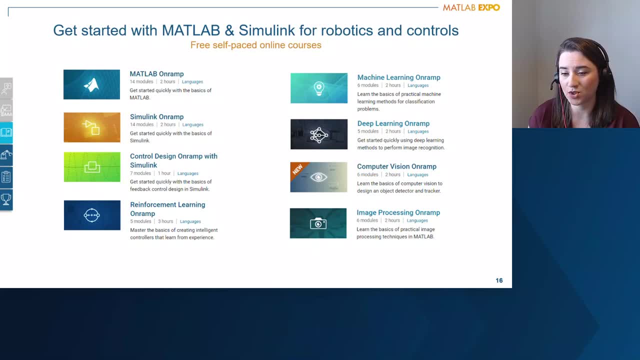 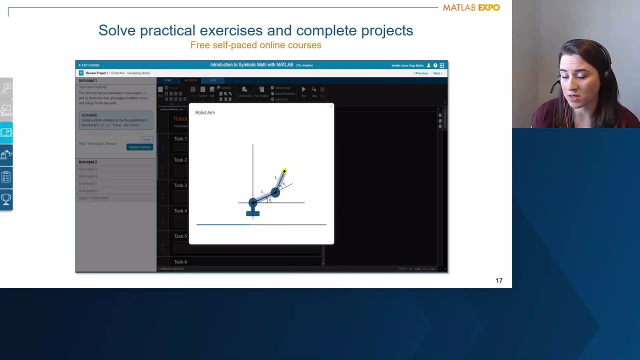 with the basics of MATLAB, Simulink control, design, AI and computer vision, among others. For the full collection of OnRamps, you can visit the link provided on the slide. The online courses can be run in any browser and contain hands-on exercises. 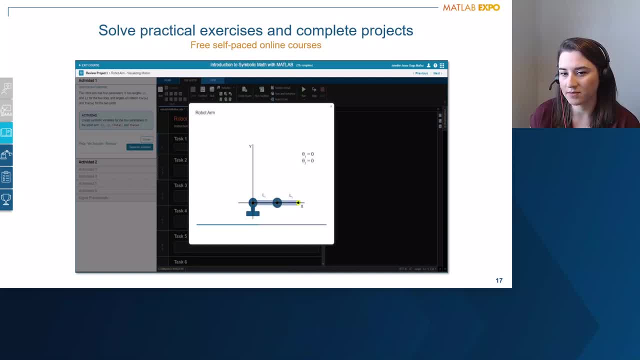 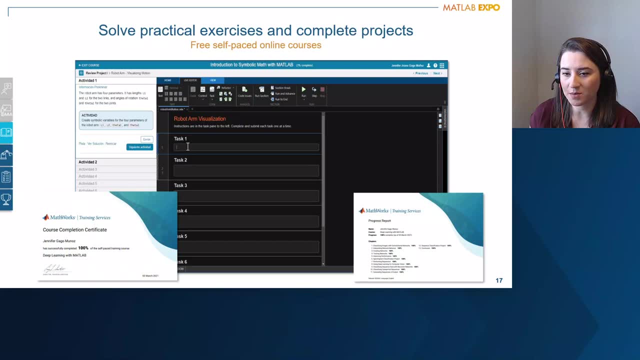 as well as short video demonstrations. Students get experience from online courses. Students get instant feedback as they complete the provided interactive tasks. They're provided with a certificate upon completion of the online course. They also get a progress report that they can share with you. 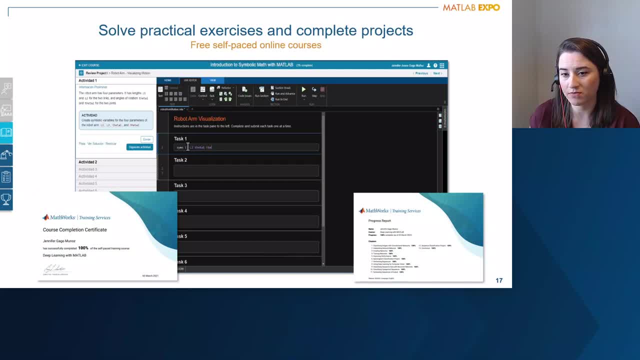 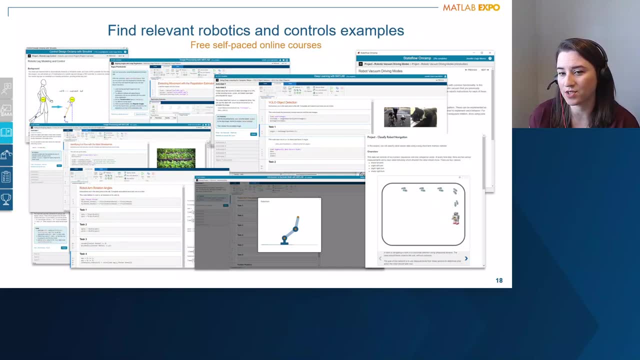 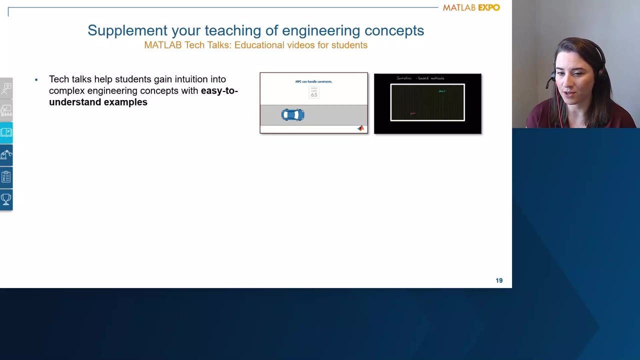 so you can check that they have successfully completed the course. All these online courses contain practical tasks relevant to robotics and control engineering, as seen on the slide. A valuable resource for students to enhance their self-learning is the MATLAB Tech Talks, a series of educational videos. 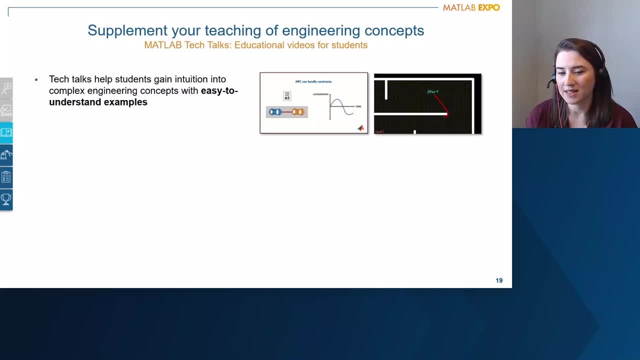 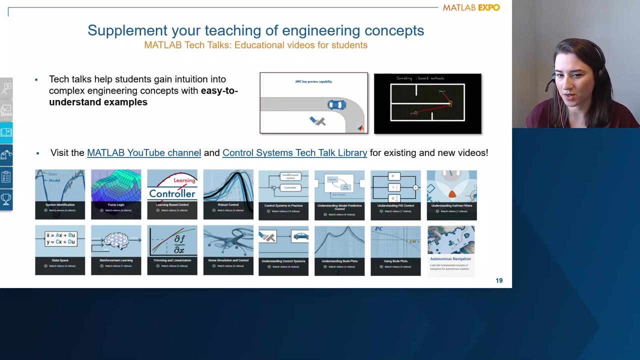 that introduce various control topics. Tech Talks use simple and relatable examples to help students grasp complex and abstract engineering concepts. With Tech Talks we cover a broad range of subjects, from PID control to reinforcement learning and from body plots to learning-based control. 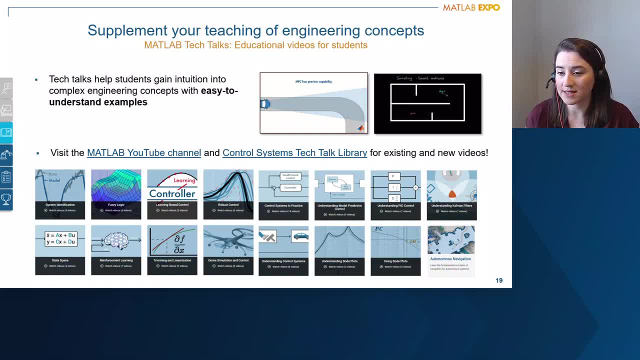 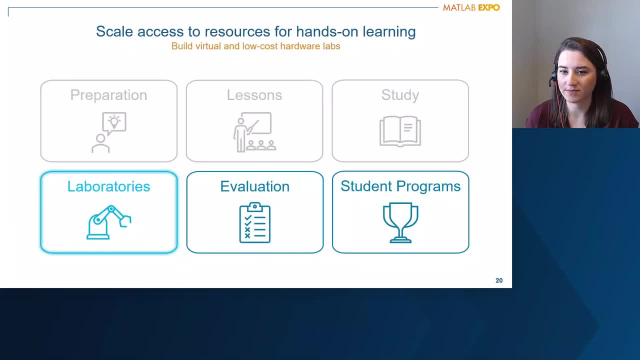 You can access all existing videos and stay up to date with new videos by visiting the MATLAB YouTube channel and our Tech Talk library. So far, we've focused on the lessons and self-learning resources for students. In the rest of this session, Jennifer will highlight the different approaches. 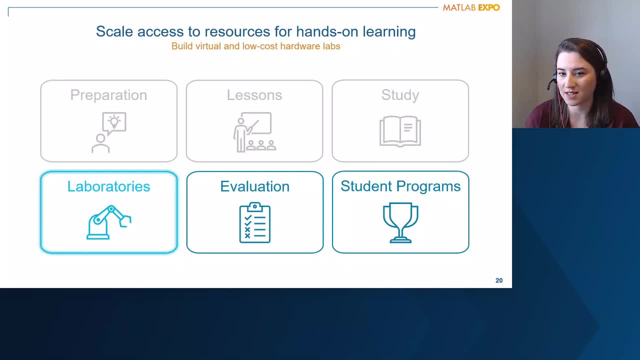 that professors can use for the practical aspects of their courses. Thanks, Mella. We know it is important to complement the teaching of theoretical concepts with applied practice of these concepts in the laboratory. One challenge with labs that we hear from professors is to scale access to resources. 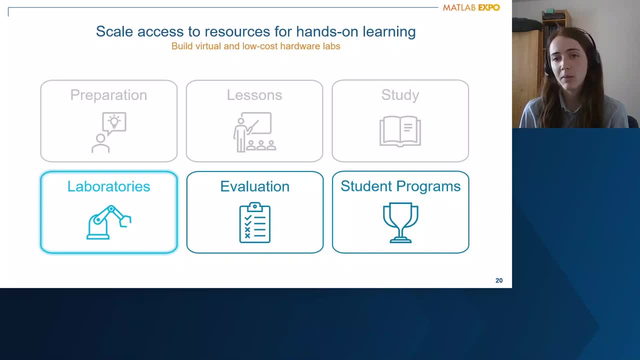 for hands-on learning, as lab activities involve hardware which can be expensive, especially classes with a large number of students. This section will show how you can overcome this challenge by using virtual labs and low-cost hardware to facilitate project-based learning, Starting with virtual labs. 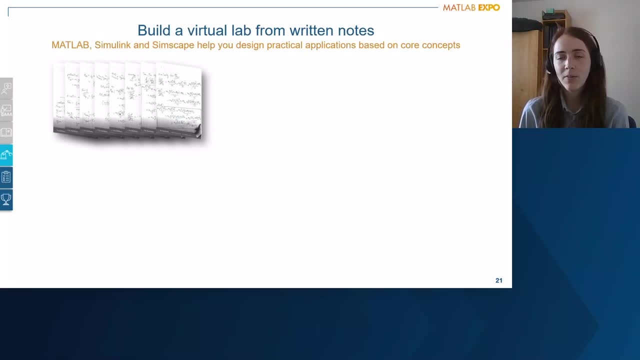 this example shows how easy it is to create a practical application from theoretical concepts shown in class. You can convert written notes on industrial robotics into a live script that defines and visualizes a two-linked planar robotic arm and calculates direct and inverse kinematics. 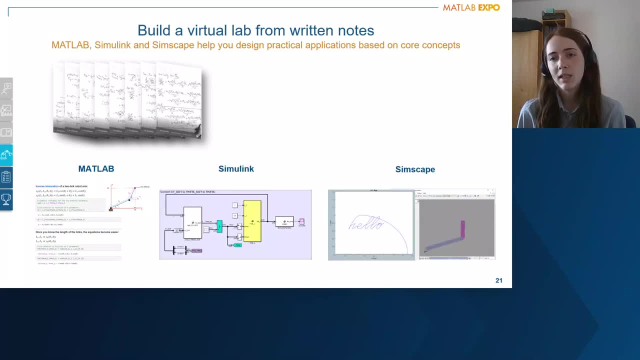 Then students can learn how to model and simulate these robotic systems using Simscape and use Simulink to understand how to use the inverse kinematic equations and the systems Jacobian to make the robot draw the world that we propose This simple hands-on application. 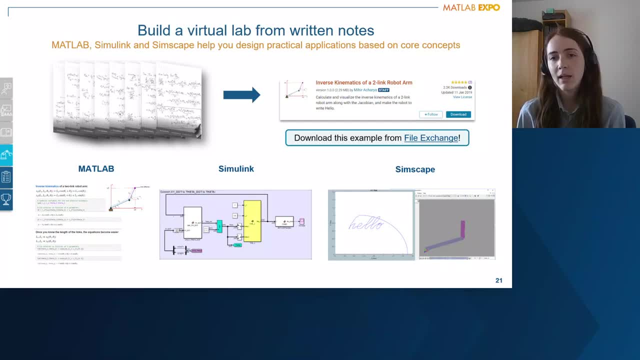 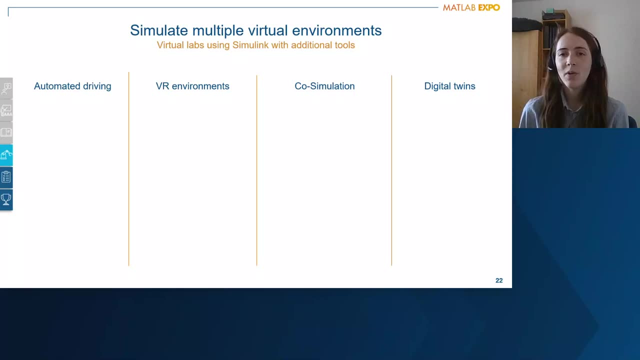 gives them a notion of the relevance of the contents explained in class to work with real applications and promotes creativity. Simulink is for model-based design as much as it is for simulation. You can use Simulink with other tools to design and simulate your systems. 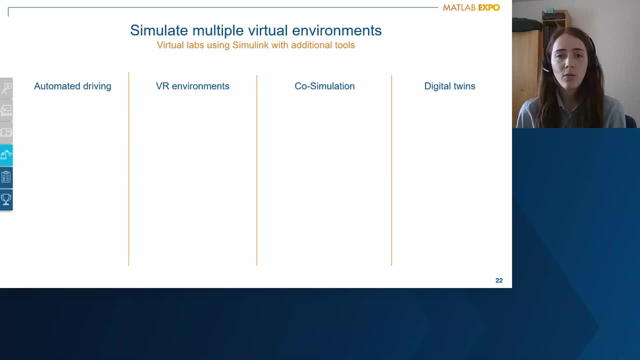 to create virtual labs or before moving to hardware. For example, you can use Simulink with Roadrunner to design 3D scenes for automated driving simulation, Or use Simulink 3D animation to visualize dynamic system behavior or robotic systems in a virtual world. 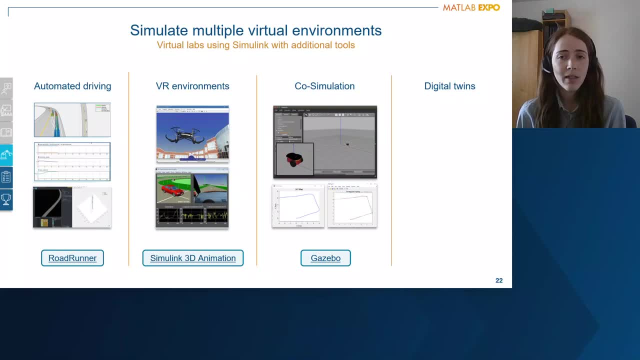 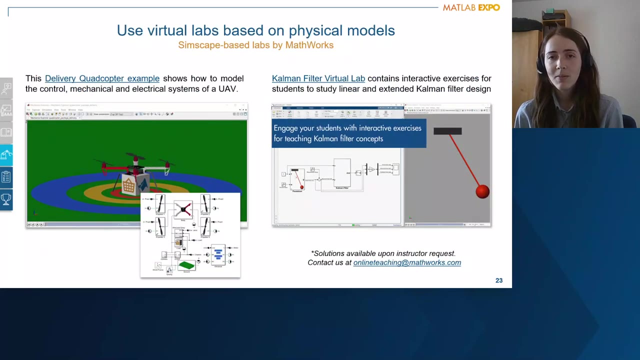 You could also set up a synchronized robot simulation between Simulink and Gachibo to send commands and receive data, Or use Simulink with Virtual Quantum Labs, which are digital twins of Quantum's hardware for teaching robotics and controls. Simscape extends Simulink. 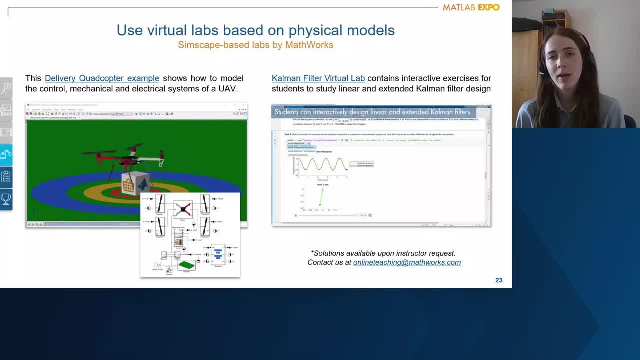 with tools for modeling and simulating multi-domain physical systems. With Simscape, you don't have to write more code to numerically solve systems of equations. You build the custom blocks, connect them graphically and let the solver do its work. 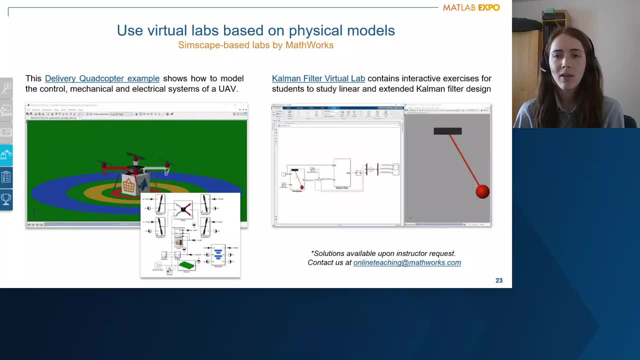 Here we highlight two virtual labs using Simscape developed by Matworks. The one on the left contains a quadcopter model that can be useful to teach students about electric motors and battery modeling, mechanical system modeling, PID control, path planning and how to use Python queries. 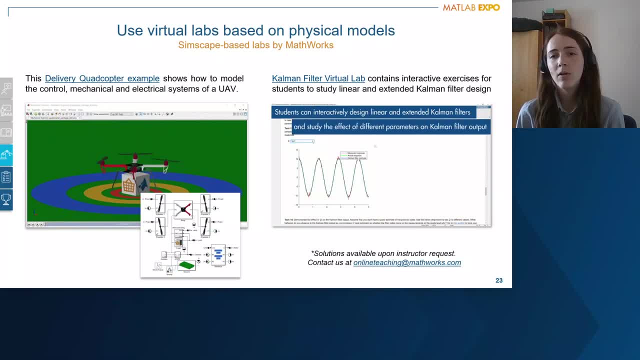 and perform a profitability analysis with Matlab. among other learning outcomes, The Kalman Filter Virtual Laboratory on the right contains interactive exercises that let you study linear and extended Kalman filter design for a state estimation of a simple pendulum system. These virtual labs let you visualize pendulum dynamics. 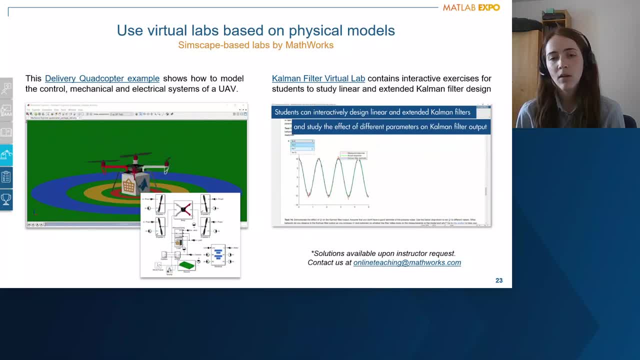 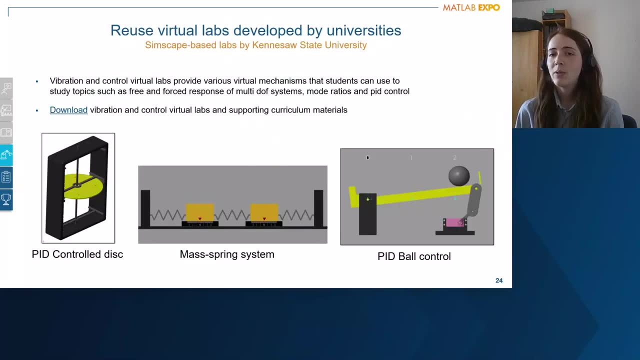 using 3D simulations and animations. Both virtual labs are available for download on the Matlab file exchange. In addition to virtual labs created by Matworks, on our coursework site you can also find labs developed by universities. Here we are highlighting the vibration and control virtual labs. 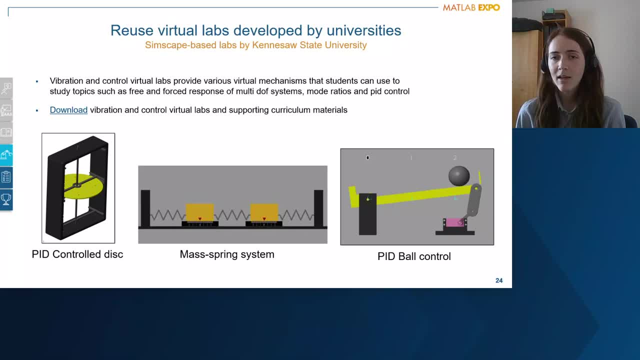 created by the Kenzo Institute at the State University. Students can adjust the parameters of different virtual mechanisms and view the system response in 3D. They can study topics such as free and forced response of single and multi degrees of freedom systems, mode ratios. 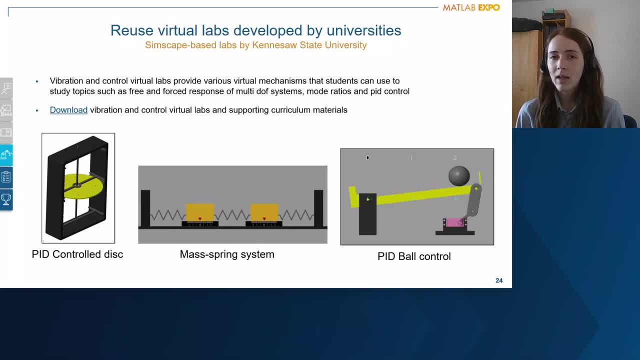 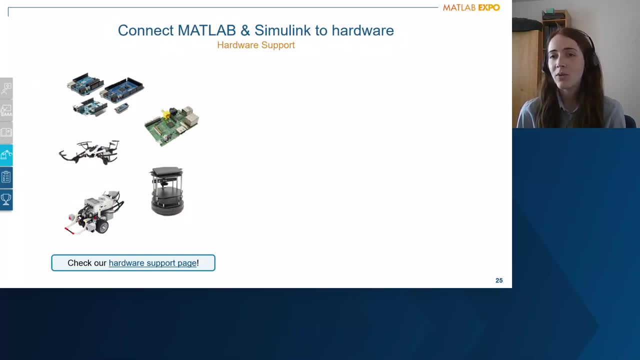 and PID control. You can download the labs and customize for your own course. Designing and simulating systems is also important to try new concepts and visualize how they will work, which keep students motivated and prepare them for a range of careers. Project-based learning. 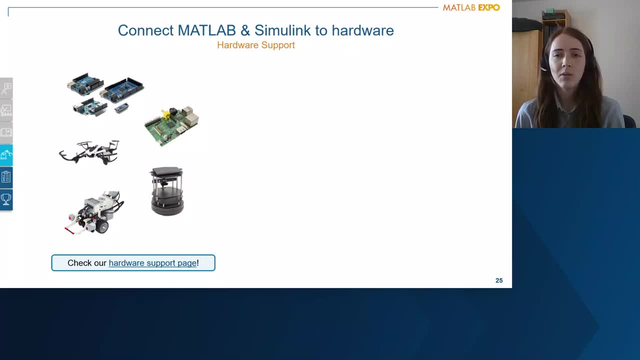 with Matlab and Simulink gives the students direct exposure to industry-standard software and hardware. Thanks to Matworks' hardware support, you can connect Matlab and Simulink to hardware such as Raspberry Pi, Arduino or TurtleBot to design test. 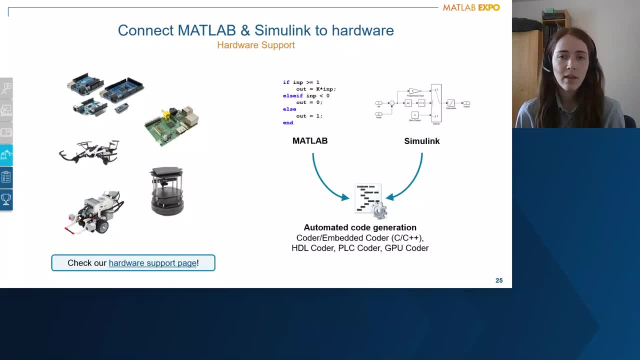 and verify robotic systems. Instead of writing thousands of lines of code by hand, you can automatically generate code to increase productivity, improve quality and foster innovation. Once you are satisfied with your model, you can automatically convert algorithms into C, C++, fixed-point. 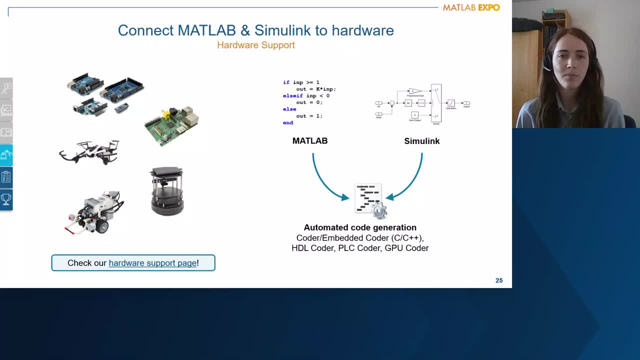 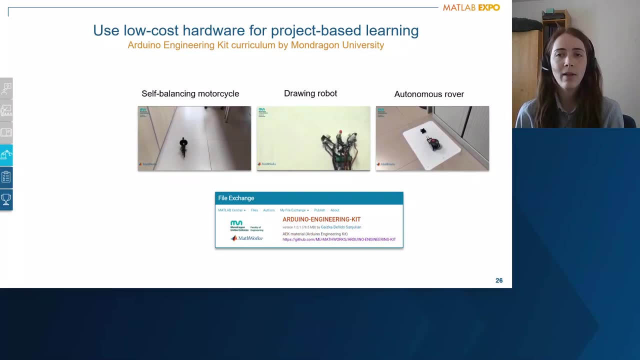 HDL or PLC code for deployment to hardware. Hands-on learning with Matlab, Simulink and low-cost hardware means students create cool projects while building valuable expertise. Working with hardware has become a foundational skill for today's engineering students. Professors from 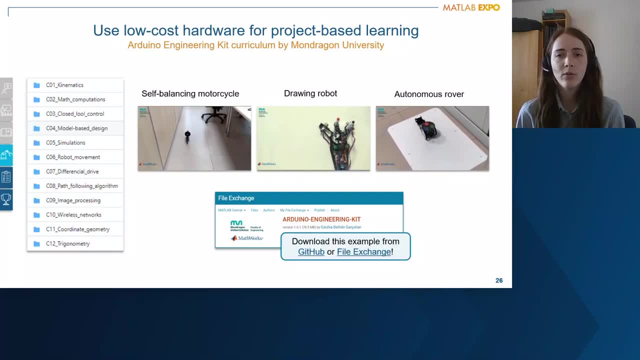 Mondragon University have built a comprehensive curriculum to cover 12 different engineering laboratory courses with the Arduino Engineering Kit. Arduino, when used with Simulink, enables students to develop algorithms that interface with a variety of peripherals and electronics for mechatronics and control systems. 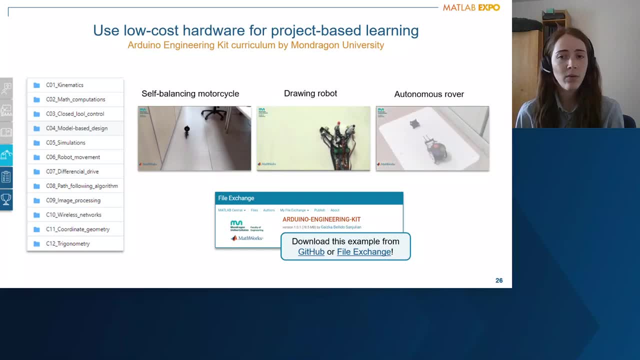 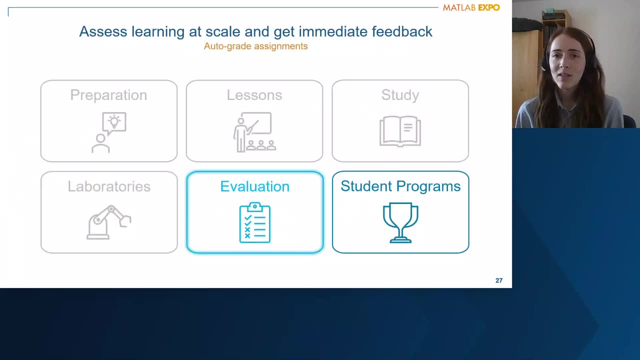 Students can develop software, implement algorithms as standalone applications and tune parameters while the application is running. Evaluation is the practical way we become aware of how effective learning is being for students. You are likely giving exams to your students that involve them designing a solution. 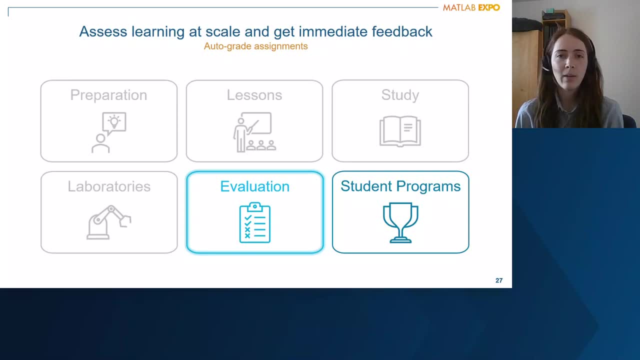 to a problem and submitting their work for grading in the form of Matlab code. But as your class size scales, you may become overwhelmed with the volume of student work to review. In this session, we'll show you how you can use autograding. 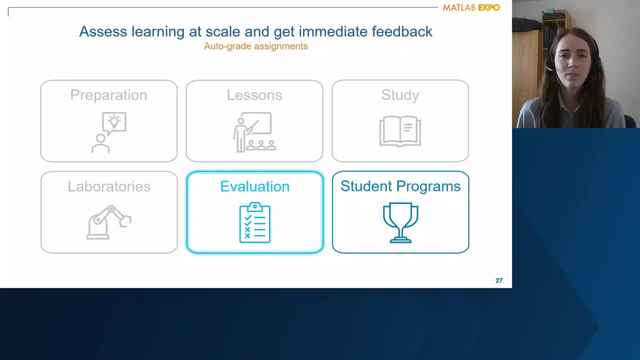 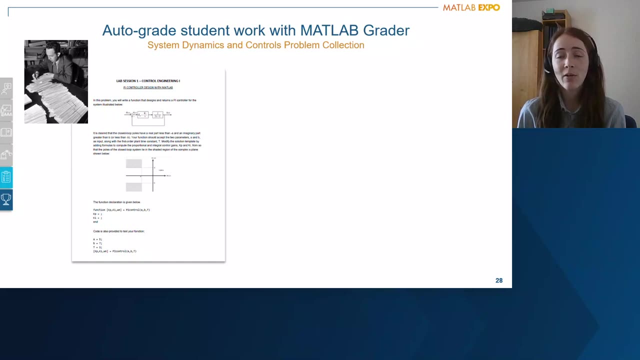 to save time and provide immediate feedback to your students on their assignments, Your desk may look something like the image on the left, covered in stacks of student responses to a last assignment, like our PI Controller example. Rather than take weeks to turn around written feedback to your students, 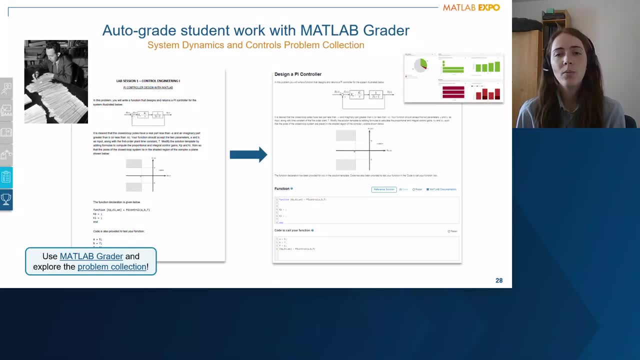 you can use our autograding solution, Matlab Grader, to convert those traditional assignments into web-based interactive and automatically graded assessments. Students get real-time feedback that they can use to improve their solutions and master the skills that you want and you get access. 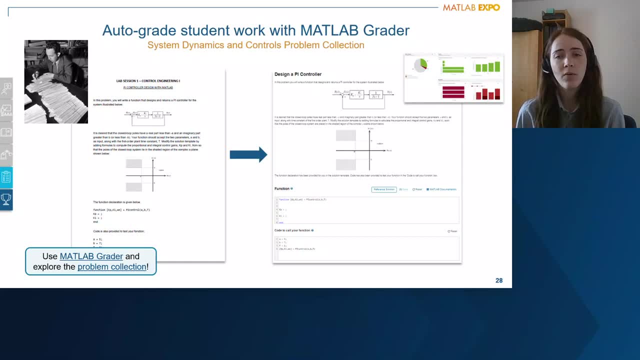 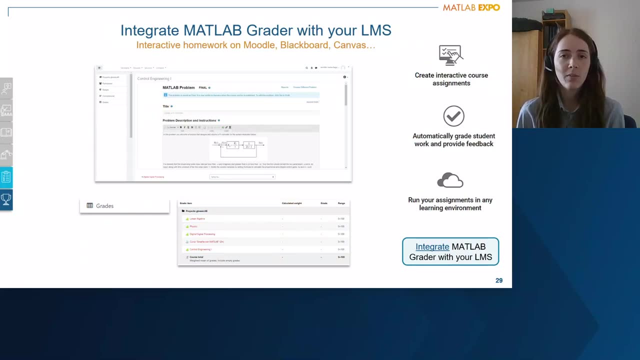 to grades and learning analytics to measure student progress and improve your assessment designs. And if you're using a learning management system or LMS to deliver other aspects of your instruction, you can add Matlab Grader to your LMS so that students are one click away. 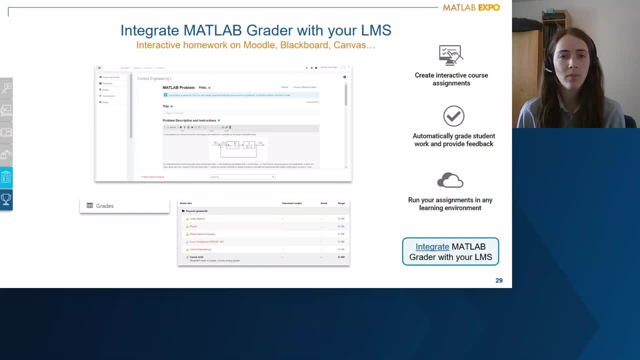 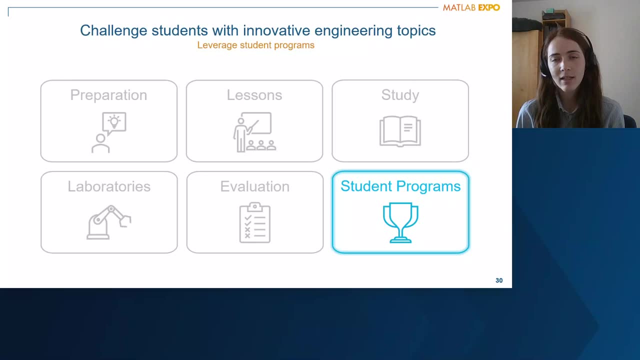 from completing their assignments and you get their grades directly into the LMS gradebook. Finally, it's important to find relevant opportunities to invite students to apply what they've learned in class, challenge them with innovative engineering topics and match their knowledge against that of other students. 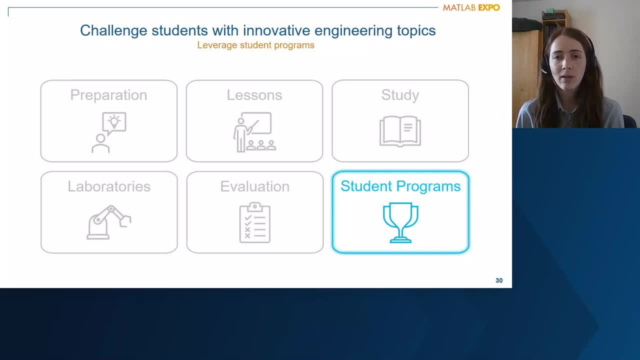 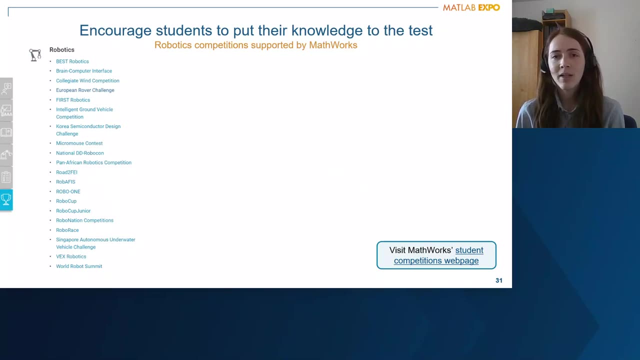 Let's explore the student programs that we can offer to our students in the future. We'll start with the Matworks and the Matworks mini-drone competition. Matworks provides complementary software training and mentoring for competitions related to robotics and controls such as the European. 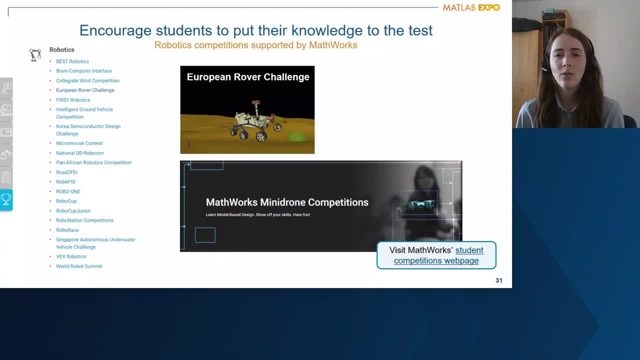 Rover Challenge or the Matworks mini-drone competition. There are also competitions related to AI or automotive, such as the Formula Student competition. Students can win prizes and bragging rights while developing their programming skills. in these disciplines, Students are transforming their accomplishments into scholarships. 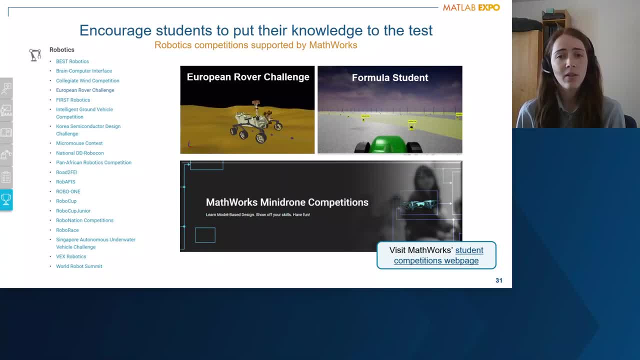 for the future. The technical and leadership skills they build during their time as a student don't go unnoticed. 70 of the Fortune 100 companies use Matlab and these top businesses are looking to hire people with Matlab and Simulink experience. In addition, 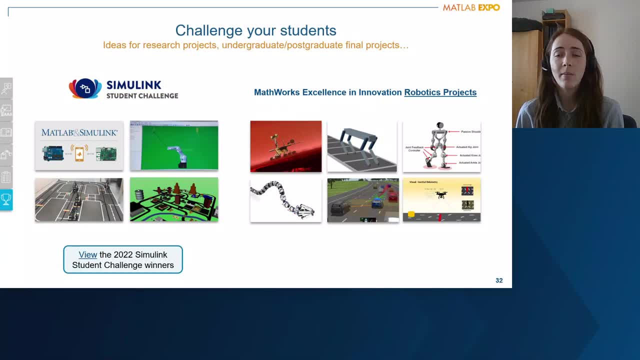 this pair of student programs are excellent initiatives to motivate students to learn about technology trends, while becoming an important contributor to the advancement of technical computing and model-based design. Simulink Student Challenge is a great way to encourage the creativity of students learning with Matlab and Simulink. 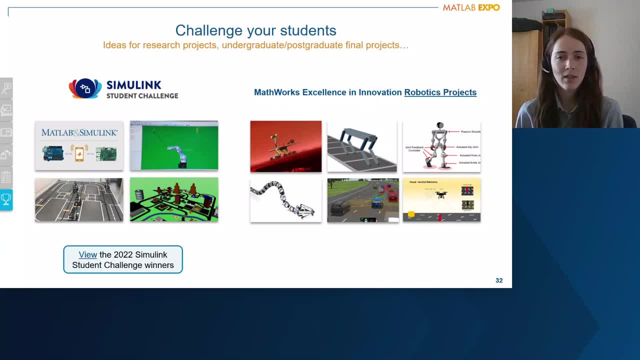 Students from around the world enter by submitting Matlab and Simulink files or videos that showcase their projects. On the other hand, Matworks' Excellence in Innovation is a list of inspiring projects based on industry trends for your capstone, senior design projects or final year assignment. 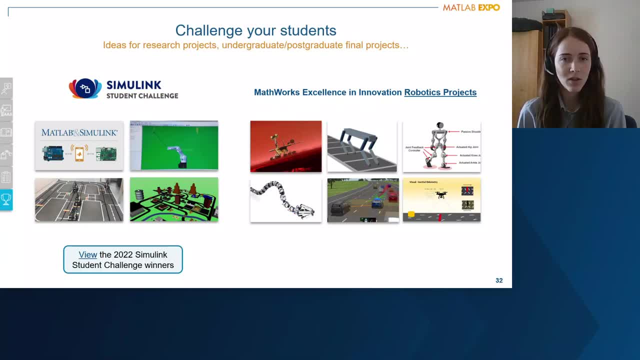 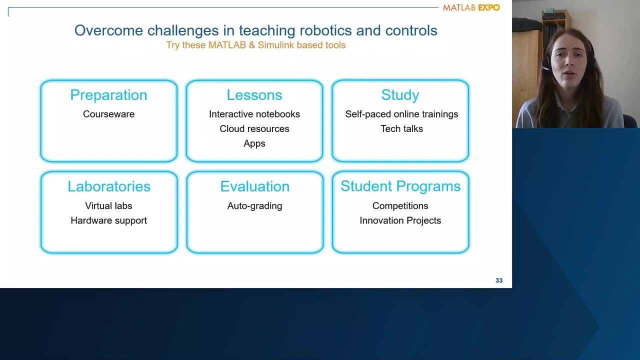 Students can gain official recognition for their problem-solving skills from technology leaders at Matworks. With these examples, we can complete the solutions shown in this presentation. We have learned how to develop a comprehensive curriculum under time constraints, with ready-to-use courseware. how to gauge. 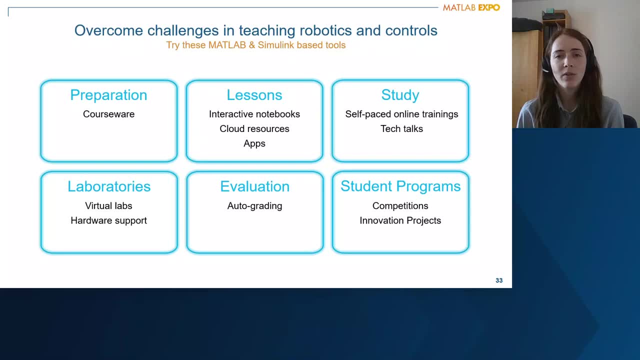 student interest during class with interactive notebooks, cloud resources and apps. how to facilitate independent learning with online training and tech talks. how to scale access to resources for hands-on learning with virtual and physical labs. how to optimize student assessment with autograding. and how to challenge. 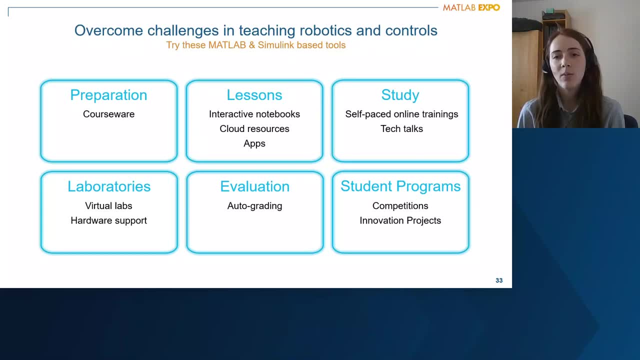 students with innovative engineering topics and solutions and innovation projects. We hope you find these solutions useful and that you can apply them to your courses, as universities such as the University of Mondragon are doing Thanks to several years of applying project-based learning with MATLAB and Simulink. 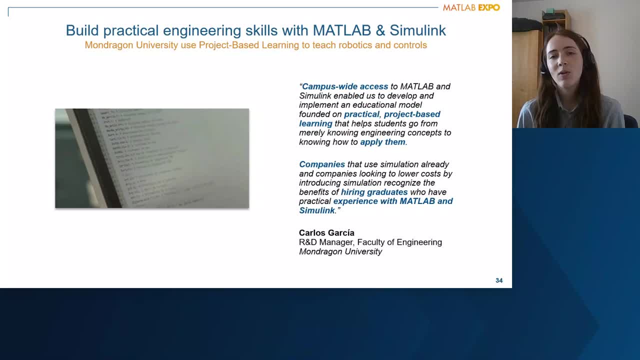 in robotics and control engineering courses, professors from Mondragon University have been able to support low-cost practical projects, increase student engagement thanks to the possibility to use the tools anywhere and anytime and receive positive industry feedback from companies that are hiring graduates who have practical experience. 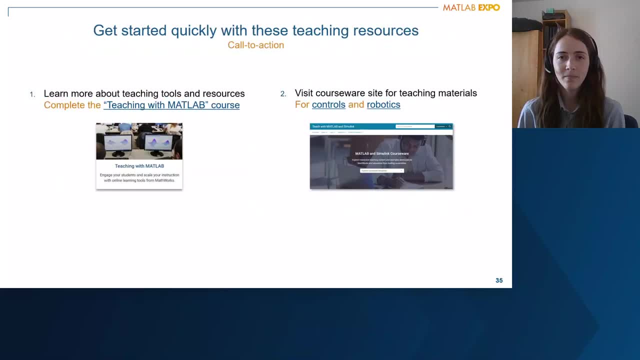 with MATLAB and Simulink. As we wrap up this session, we want to leave you with a couple of call-to-actions. We encourage you to take the Teaching with MATLAB course, which helps you create engaging and scalable instruction with MATWORKS online learning tools. 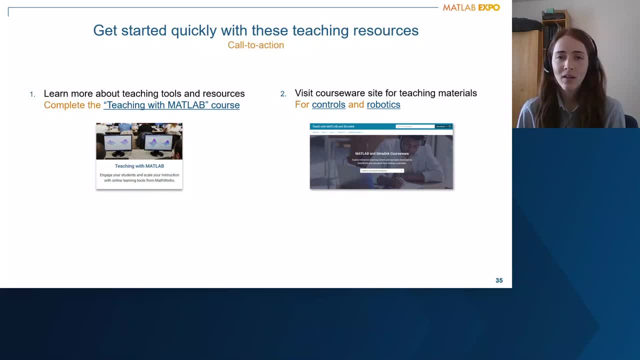 Today we talked about various control and robotics curriculum materials developed by both MATWORKS and different universities. To find those resources and much more, please don't forget to visit our MATLAB and Simulink courses If you are creating a new control or robotics curriculum. 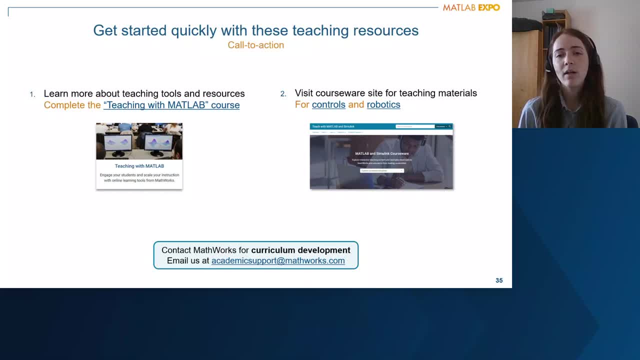 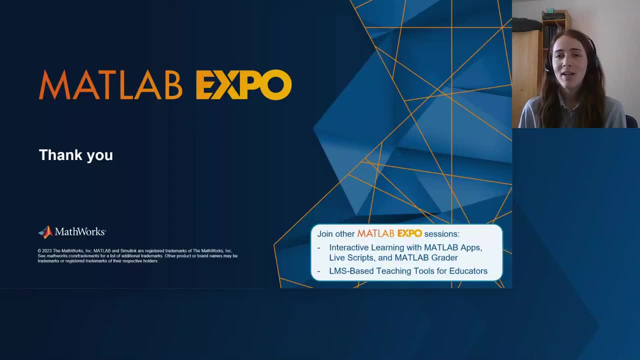 and want to learn how MATWORKS supports curriculum development. you can contact us at the provided email. Thank you for joining us for this MATLAB exposition. If you found this content interesting, you are sure to enjoy the following sessions on interactive learning and LMS-based tools. for educators.